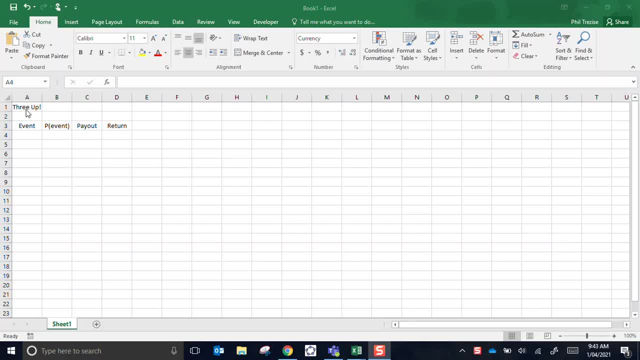 you throw three coins in the air. Now I have to decide. I'm going to do some theoretical calculations here. I have to decide which events are going to be winning events Now. I think if we get three heads, that should be a winning event. I also think if we have 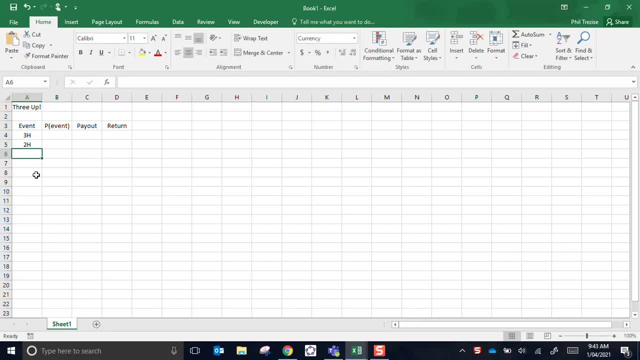 two heads. that should be a winning event And everything else will be a loss. So that would be one or zero heads showing up. Let's just type that a bit better so that it fits neatly: One head, zero heads. I still need to do this. I'll just make that column a bit wider, so. 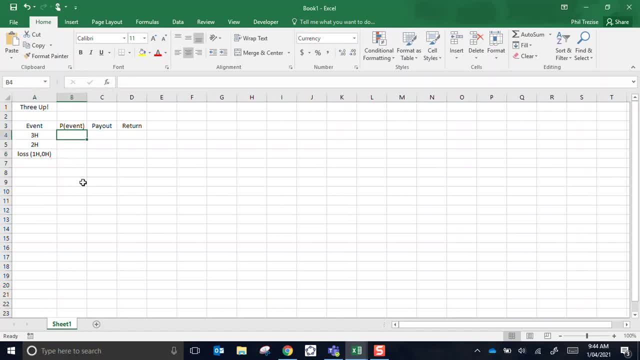 it fits nicely. Now, as this is a very simple game, I can work these probabilities out straight away. The chances of getting three heads in a row. well, there's only one way that can happen: if all three of them turn up heads, And the chance of an individual coin landing. 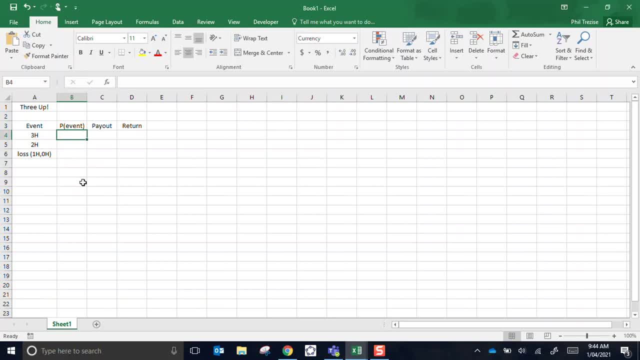 on heads is a half. So a half times a half. A half times a half is one eighth or 0.125.. That shouldn't be money, That should just be normal old numbers, please, And let's have a slightly. yep. there we go. Now what about? 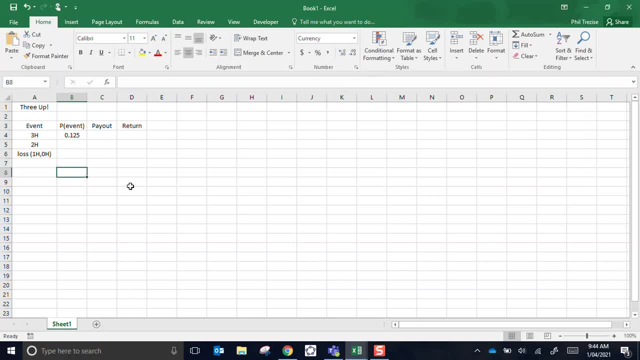 the chance of getting two heads. Now this is where we have to start thinking about combinations. How many different ways could the coins land if, of the three coins I'm choosing, the first two of them are heads? So 3C2, that's three, And each of the outcomes is a half times a. 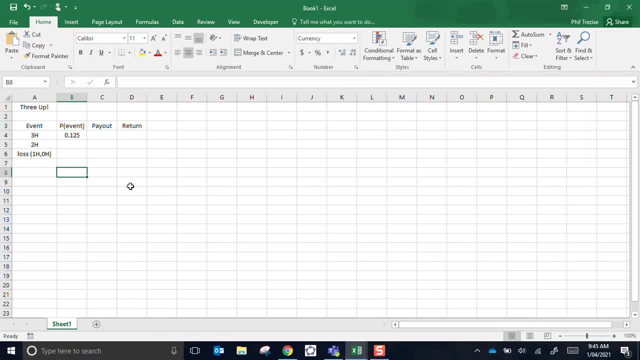 half times a half. Whether it's a head or a tail, it's a probability of half. So it's basically three times that number there 0.375.. And again, somehow that's turned into money. Let's have that as a number, please. Now, what are the chances of getting the other? 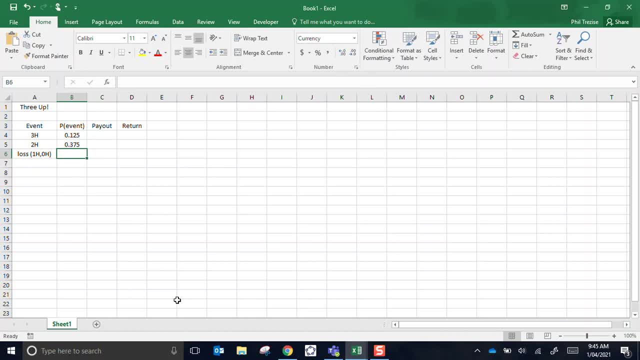 outcomes. Well, it has to either be three heads, two heads, one head or zero heads when you throw the three coins. So the losses are the complimentary event. If you add these two, you'll see they come to 0.5.. So that means that it's a 0.5% chance. For some reason, everything in my 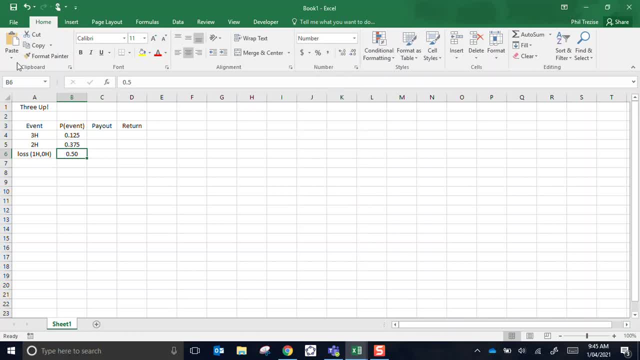 spreadsheet thinks that it's money. That's annoying. Let's just do this and make sure that everything is just a general format. So that's good. OK, Now we have to decide the payout on these different outcomes. I'm going to assume that 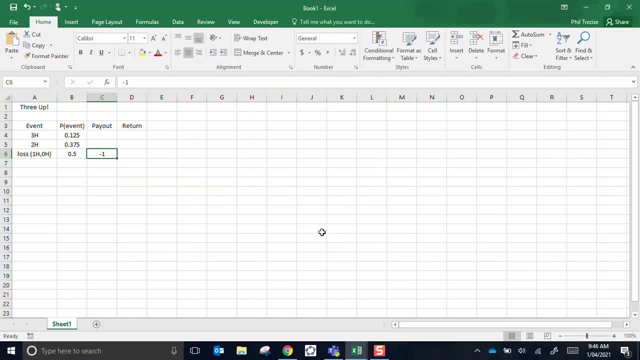 the players make a $1 bet. So pretty much. and this one could be money, couldn't it OK? So if the players make a $1 bet and they lose, then their payout is negative $1. The casino keeps the money, But let's make some. well, I'm not sure exactly what these ones will. 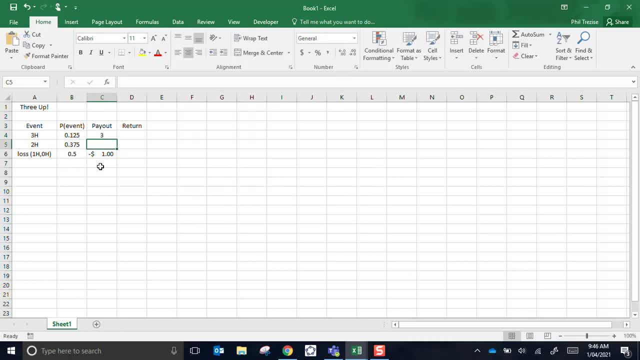 turn out to be. Let's give this one what they look like. Here we go. I'll hit the minus surprise of a $3 payout, and let's give this one a $2 payout Again. I'll make those ones into money. 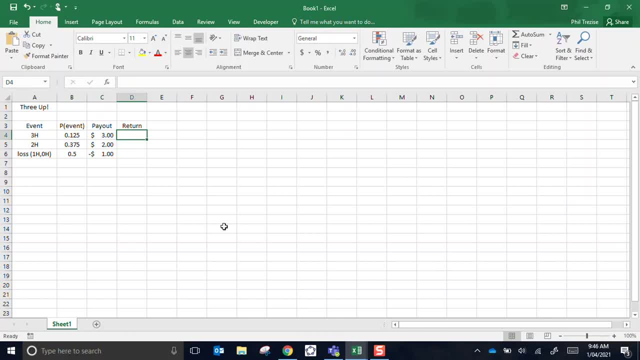 Now the return to the gambler. Well, that payout only occurs. we expect one turn out of every eight. So the return to the gambler is the probability of the event multiplied by the size of the payout. So on average we would expect that occurrence, the three head event, to give. 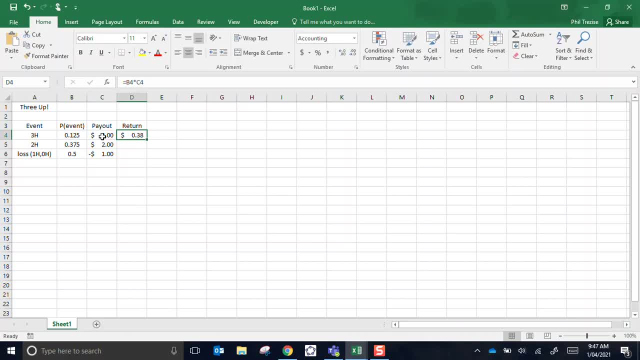 a payout of $0.38 to the player. Likewise, for this one we'll go this number multiplied by the $2 payout, So that's actually going to be a more profitable event. The player, because it's only a $2 payout, but because it occurs much more often. 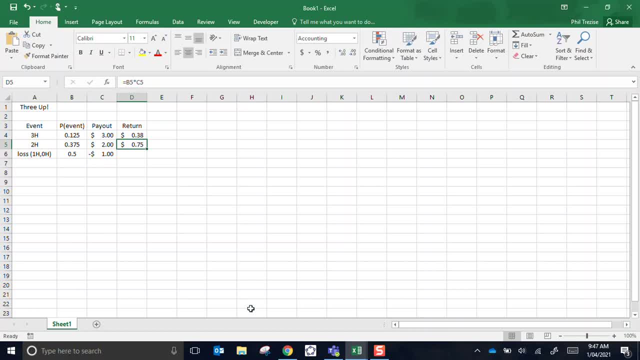 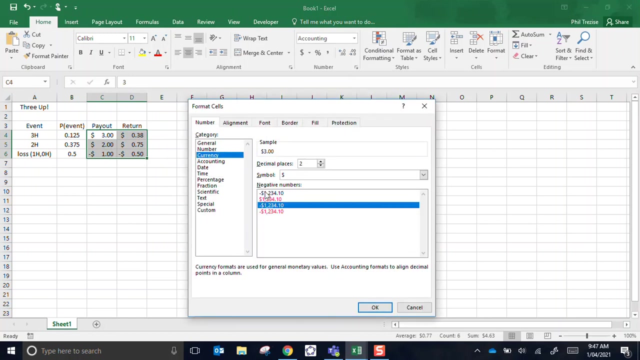 on average, that event pays $0.75 to the player. And lastly, we'll do this one multiplied by this one And we get that. Now, these things that are money. I would just like to format those. If I put currency, I can format the negatives to be in red. It just makes them stand out a bit. 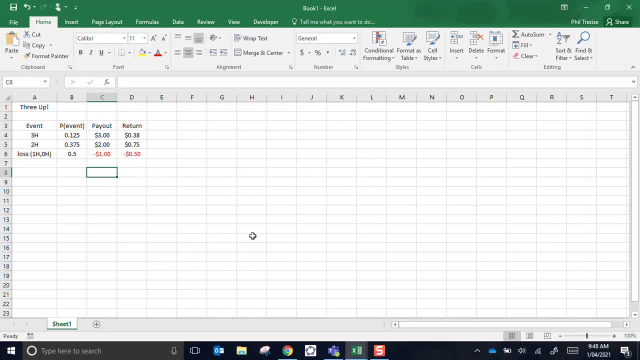 Now what is the? this is the total return to the player. then I'll have the sum of these numbers. Now, that's good for the players because it's a positive number On average. the player is going to get a payout or a return of $0.63 every time they play the game. That's not good for the casino. 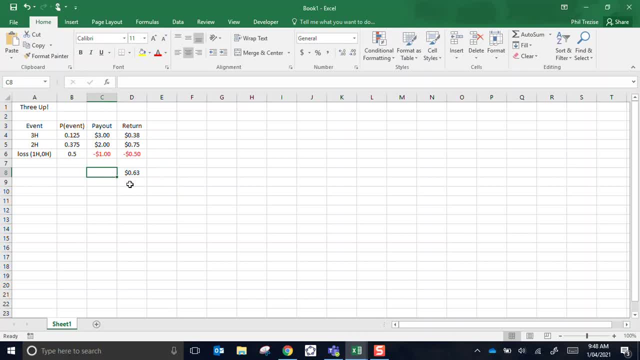 What that means is I need to lower the size of the payouts for the winning outcomes. I'm paying too much. What if I paid $2 for this one and $1 for this one? Now that's still going a positive return to the player. I'm still have prizes that are too much, So maybe I could lower this one to $1.50.. 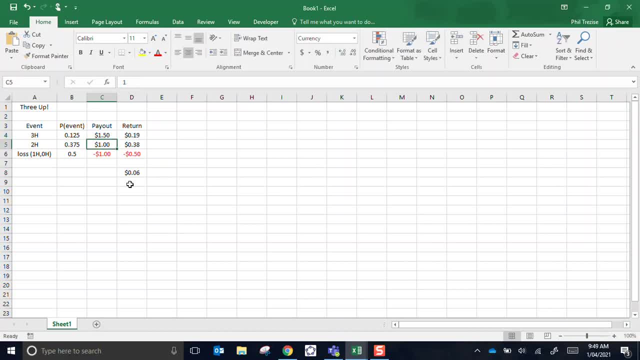 Sorry, that was supposed to be $1.50. And this one could be $0.75. So that's what we're going to lower this time. I think that's a real big way of doing it. Now, this is the functions that we're going to use. 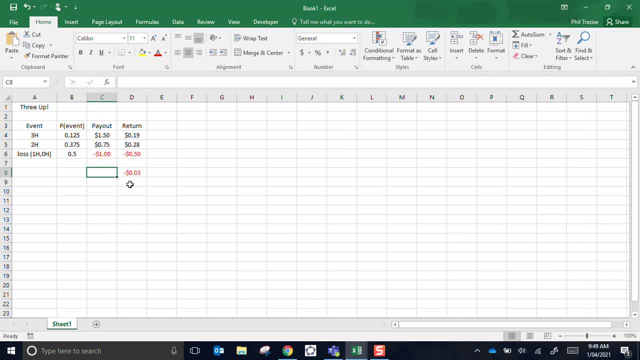 So this is the POS movements And this is the aireKorean W? mm-hmm, this is w restore pays. this one's a wait, so it's going to break the. if that's the trade, I'm going to let Eminence the return to gold sex. 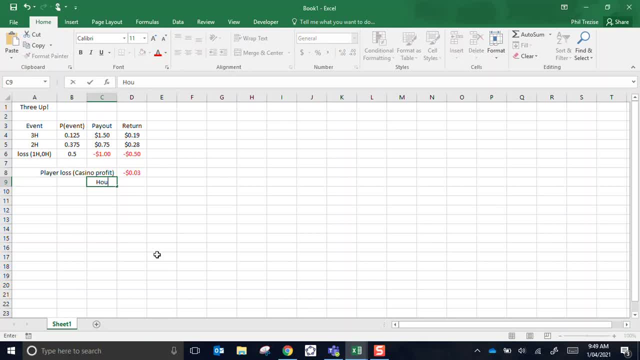 So what you would want, you know, is bottom. Now, what about the house edge? The house edge is literally how much the house collects or wins- in this case, $0.03, compared to the amount the player bet. the player bet $1. 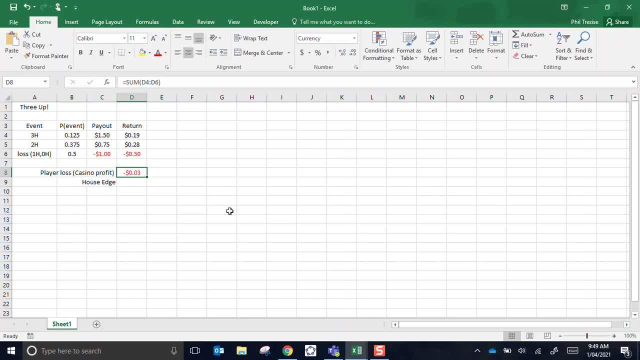 So that is literally a 3% profit. I will go negative 1 multiplied by that number. so it's now a positive number and I'll format that as a percentage and I might give one extra decimal place. Now a 3.1% house edge doesn't seem like very much and it's not for an individual game. 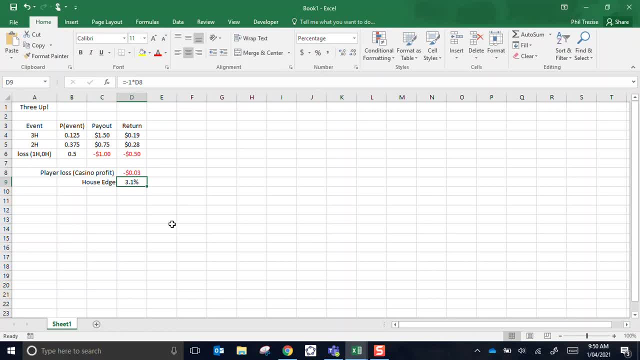 But if we can convince people to play thousands upon thousands of these games, then this will actually end up being a very profitable outcome for the community Casino. In the long term, they'll collect 3.1% of all the money that gets bet playing this game.